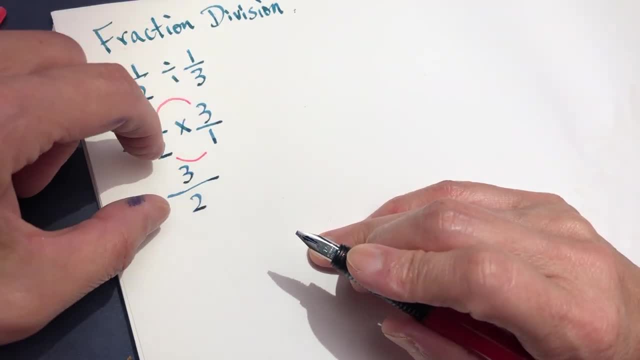 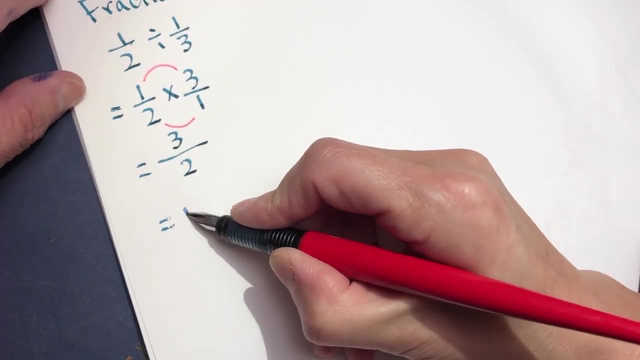 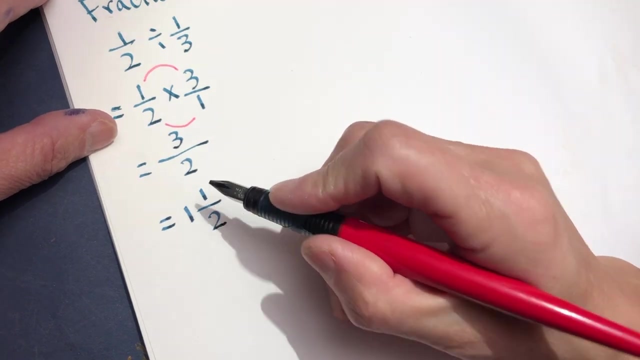 in high school. Some teachers prefer pure fraction And some teachers, especially in elementary school, they would like to do it with mixed number form. So one over one and one over two. one and a half: Okay, this is our first problem. 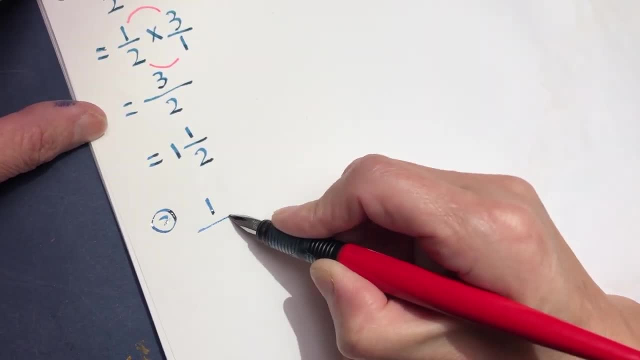 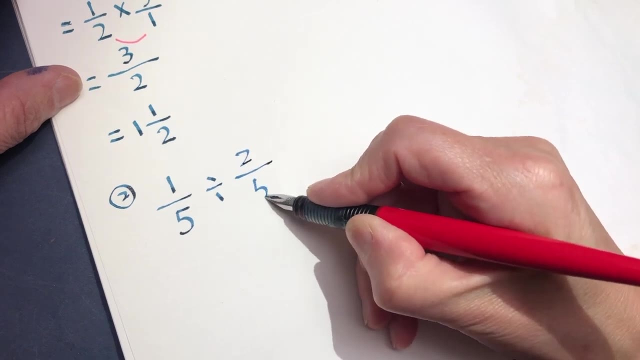 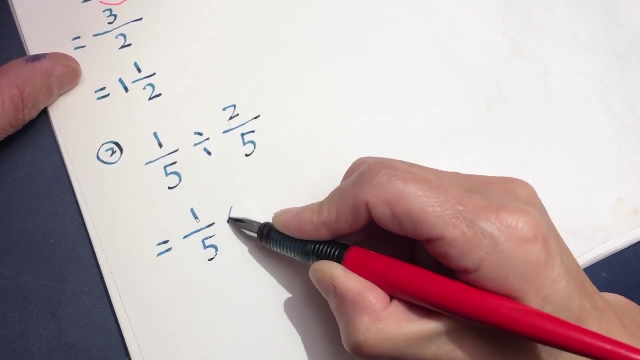 Now we do the second problem: One over five. divide it by two over five. So this one first number never change. Second number upside down: five to the top. Two over five. one over five. So this one first number never change. Second number upside down: five to the top. 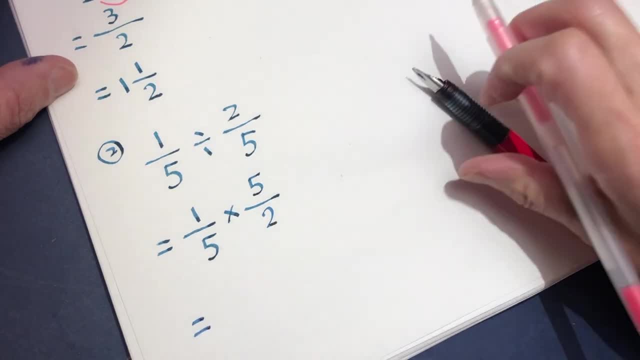 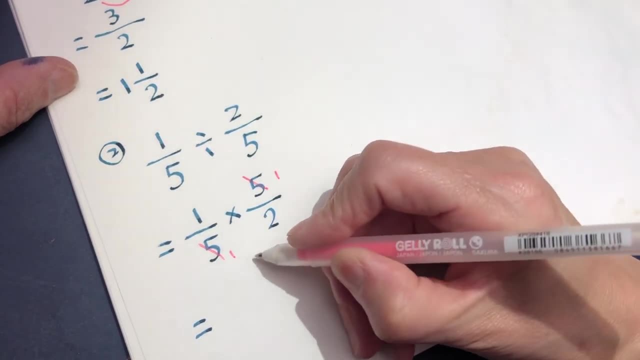 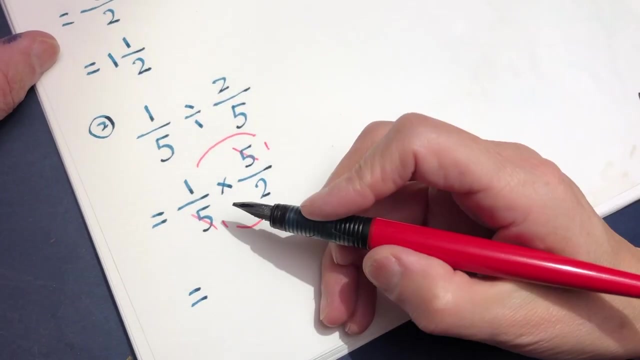 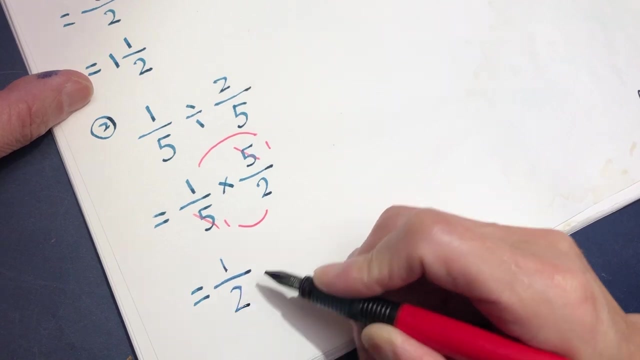 two to the bottom, and here we can simplify five, and five can be cross-canceled, and one times two, one times one with our glitter pen. so one times one is one, one times two is two, so the result is half. 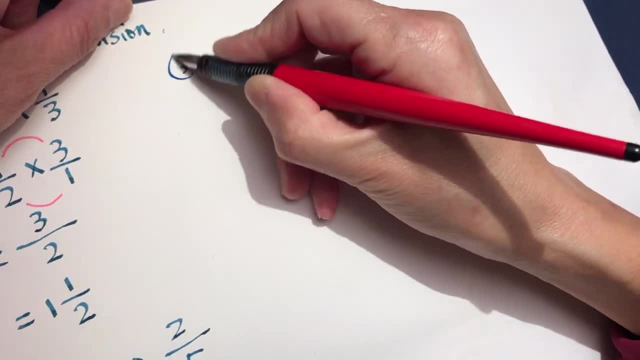 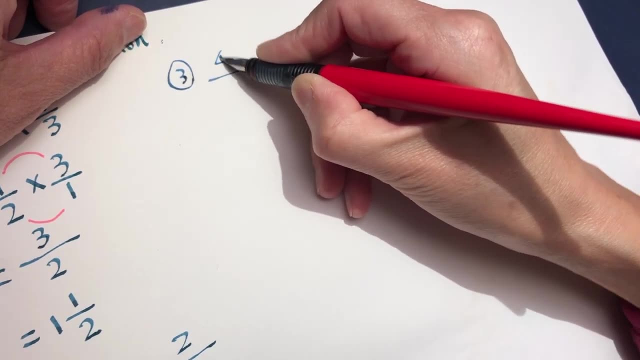 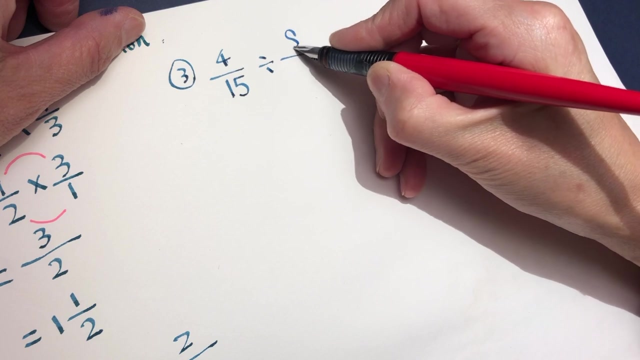 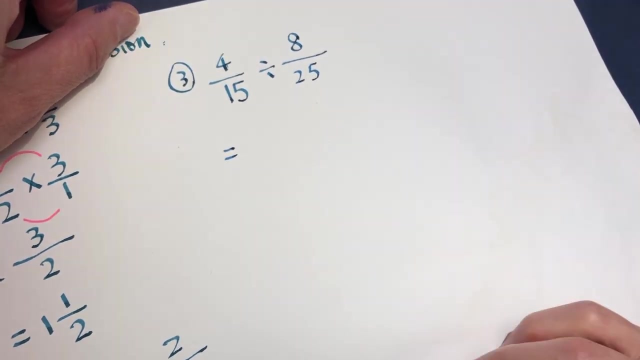 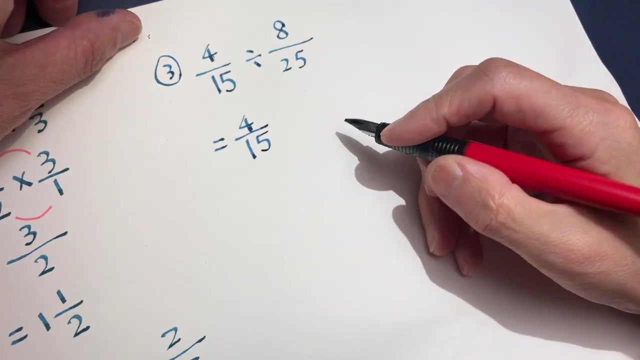 Okay, now we make the number a little bit more interesting and more complicated. So four over fifteen, divided by eight over twenty-five, Let's do this So four, we do not change. four over fifteen, the first number, never, ever, ever, never change. 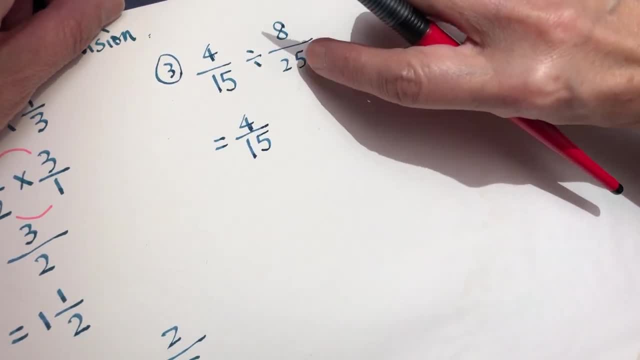 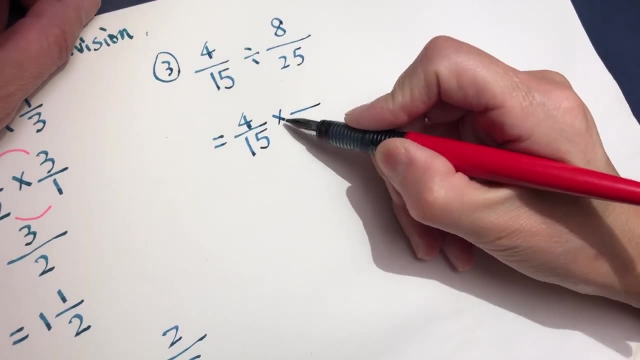 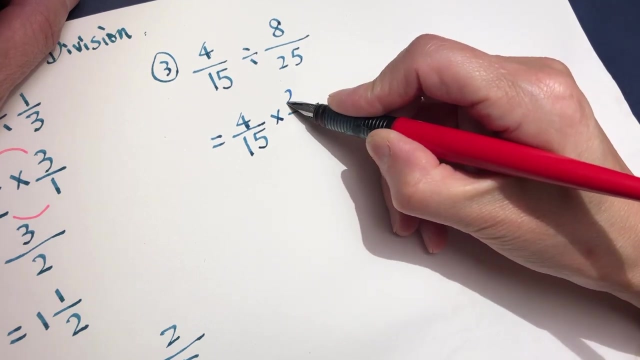 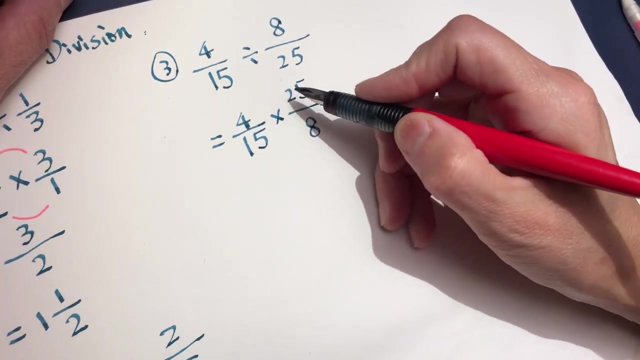 and the second number, the dividing number, the divider. we will change it upside down to make it into a multiplication form. So the bottom is twenty-five now we move it to the top. twenty-five over eight. you can do the multiplication. 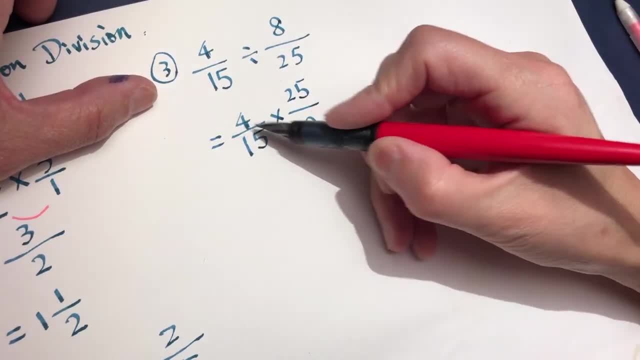 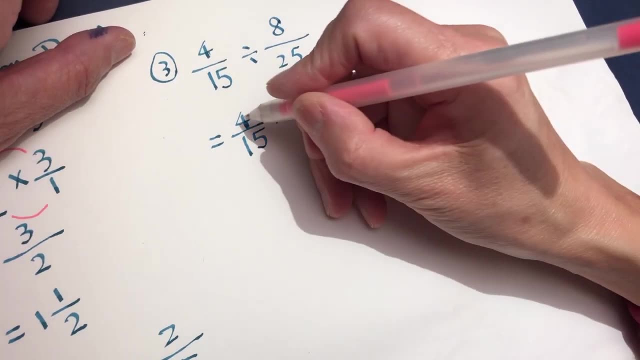 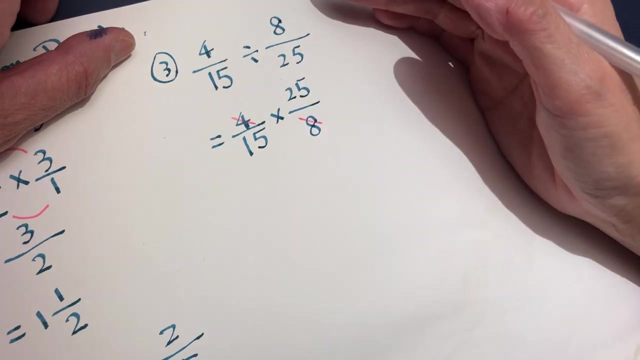 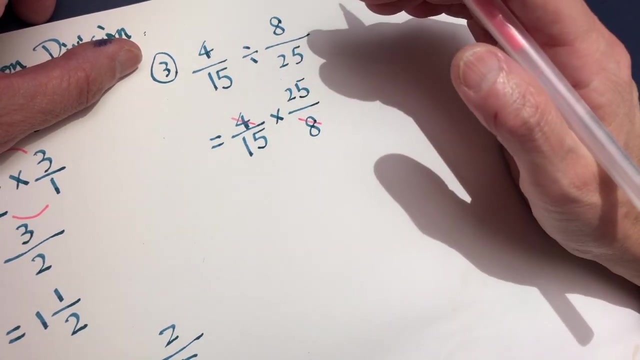 but the number is twenty-five. it's too big. why not simplify at this stage? When you do math, one of the core values in math is to simplify as early as possible or make your calculation as simple as possible. Do not allow a lot of big numbers without simplifying. 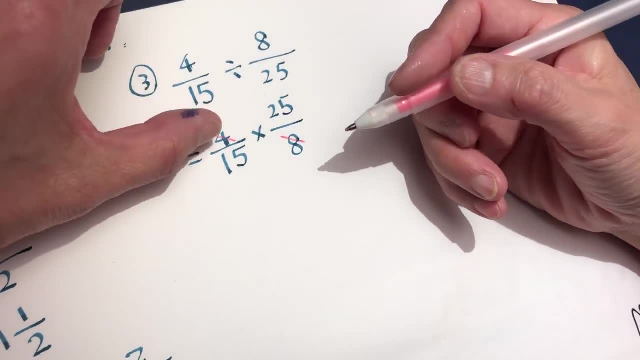 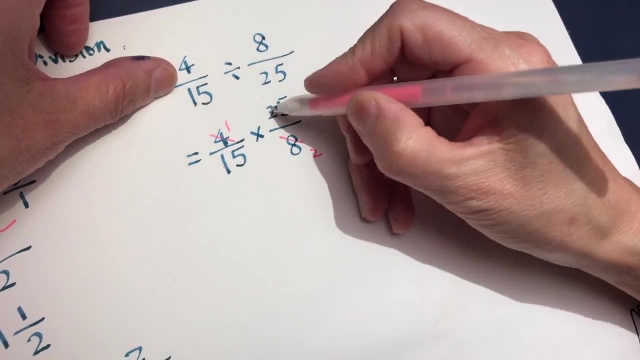 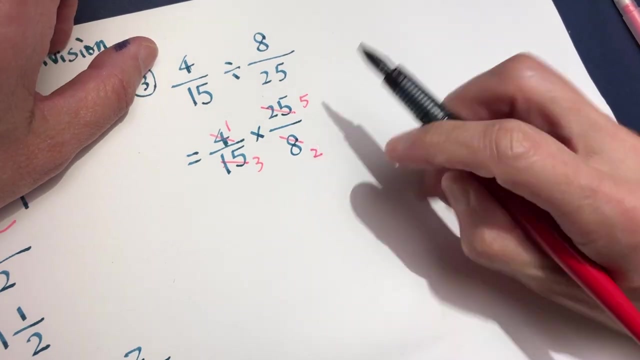 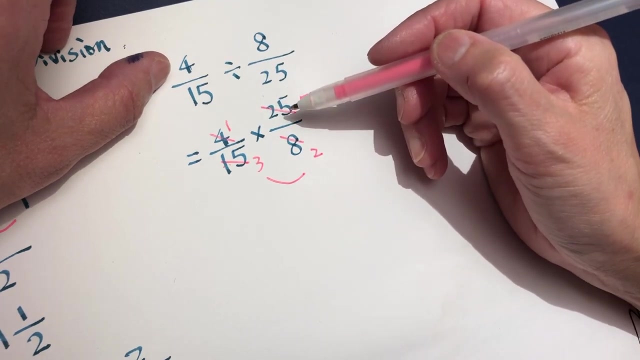 it will increase your chance to make mistakes. When you both divide it by four, it's one and two, both divided by five, five and three. So this way, three times two is much easier than fifteen times eight, Four times twenty-five, although you know it's one hundred. 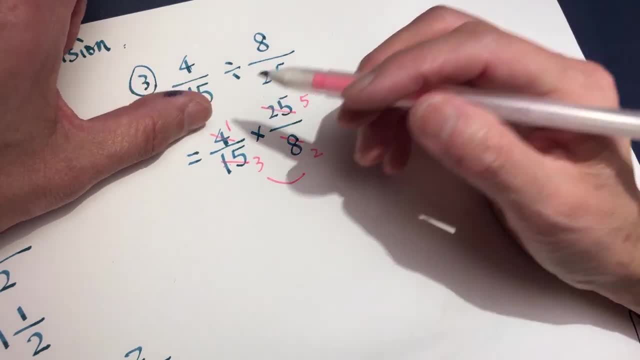 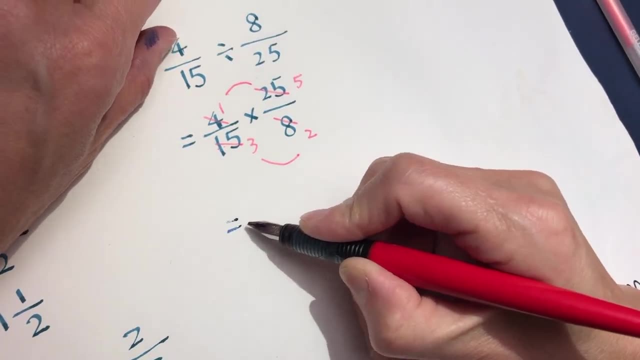 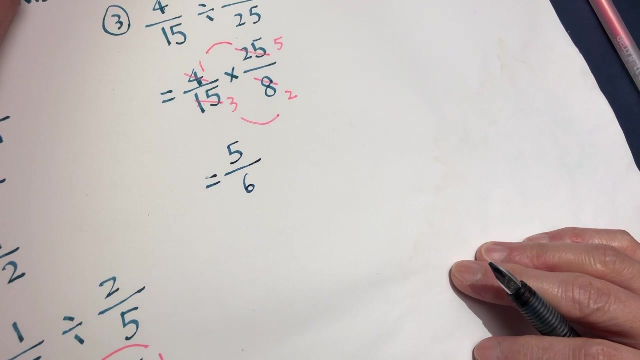 four quarters makes one hundred. but still, one times five is so much, It's so much easier, right? One times five is five, three times two is six. Easy peasy, lemon squeezy. Okay, number four: we make another problem. 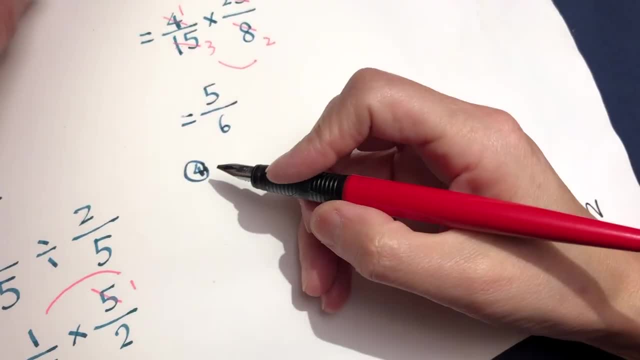 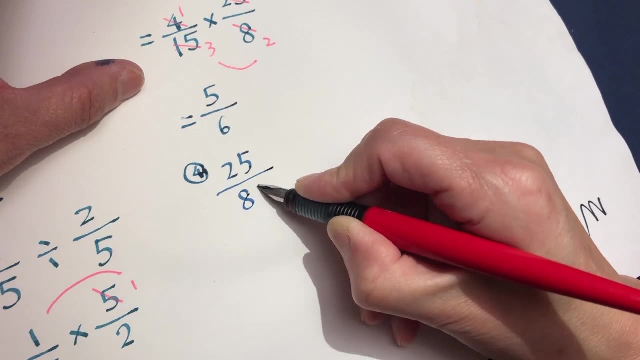 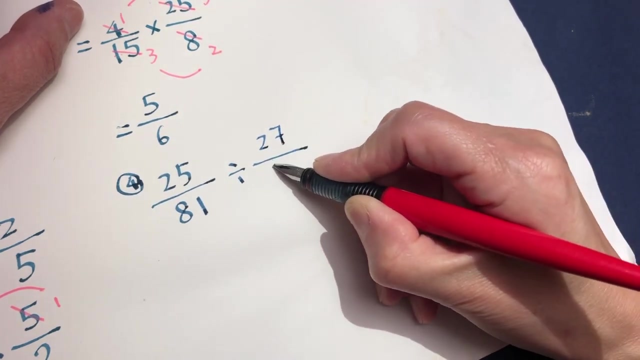 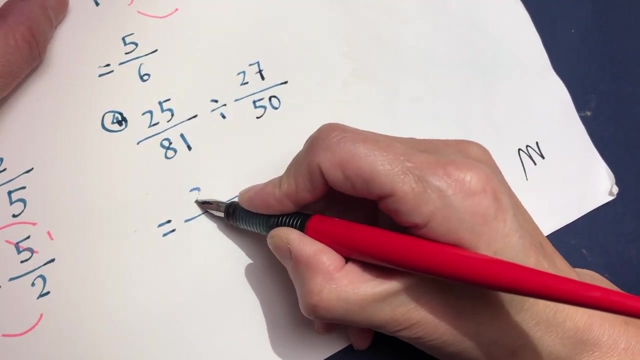 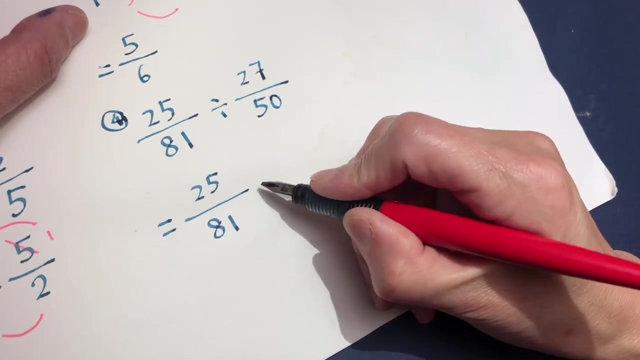 Too many numbers? Okay, this one with twenty-five over eighty-one, divided by twenty-seven over fifty. So, first number, we do not change twenty-five over eighty-one. The second number, the divider, we will change the sign from division to multiplication. 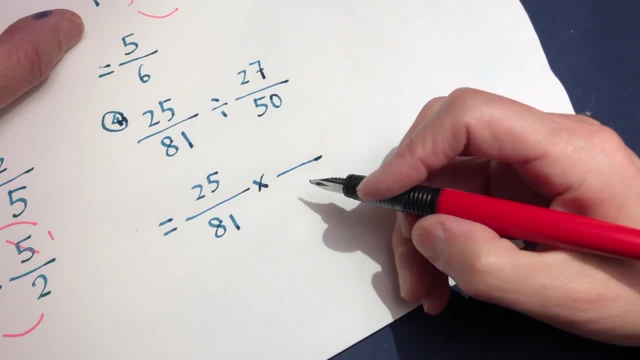 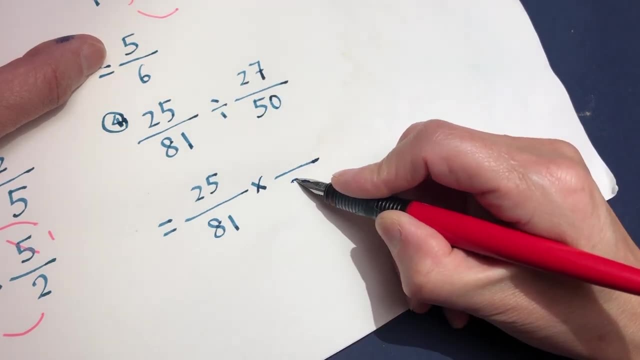 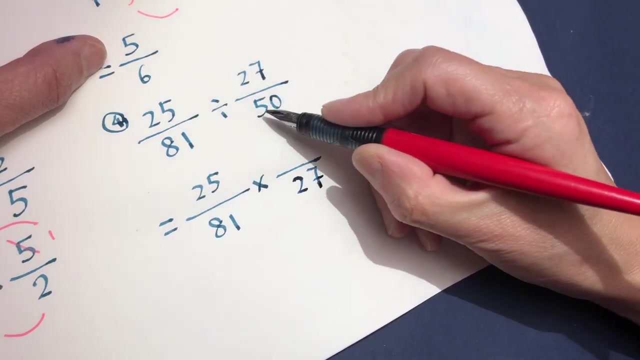 What do we do on this side? We will flip it up. okay, So twenty-seven on the bottom. we will move it to the on top, move it to the bottom. twenty-seven and top is fifty, the bottom is fifty. 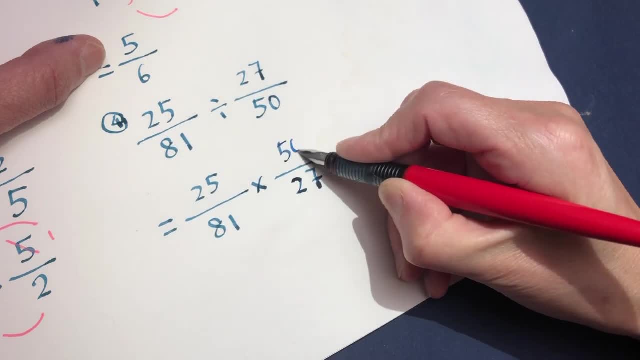 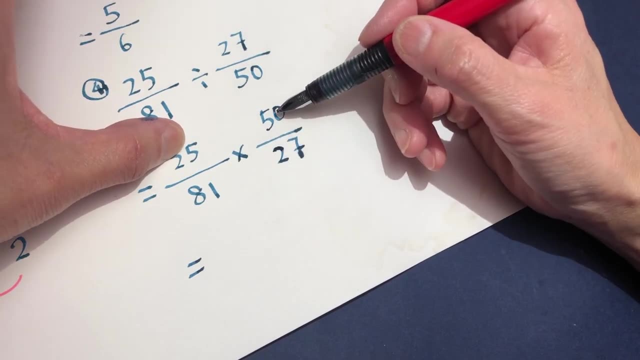 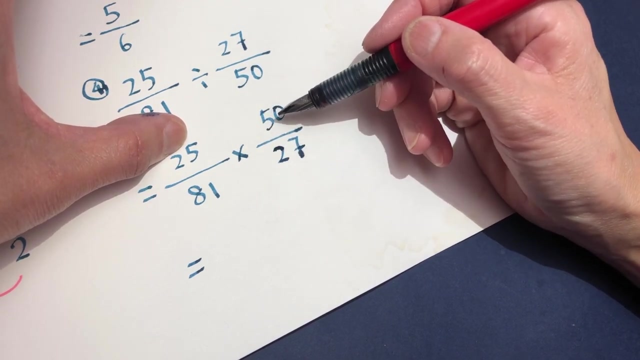 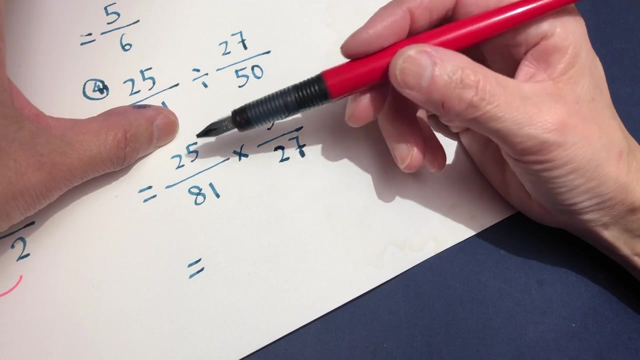 now we move it to the top is fifty. Okay, So twenty-five and fifty. Oh, this is one. this is two times fifty. Can we cross cancel? No, I intentionally made this problem, Not really intentionally. Anyway, I realized that they are both on top. 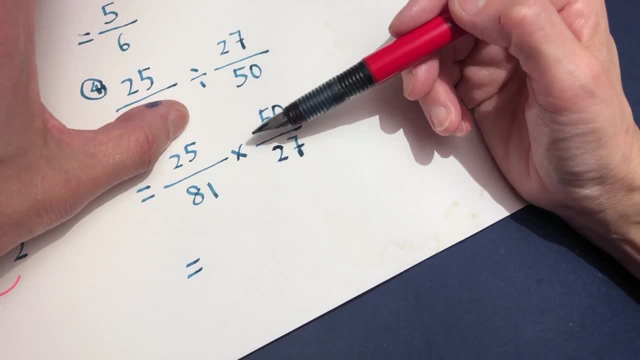 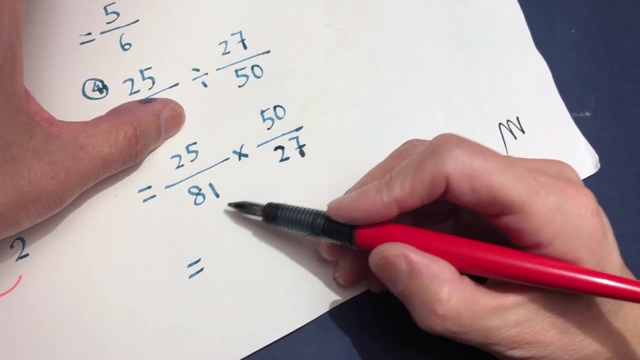 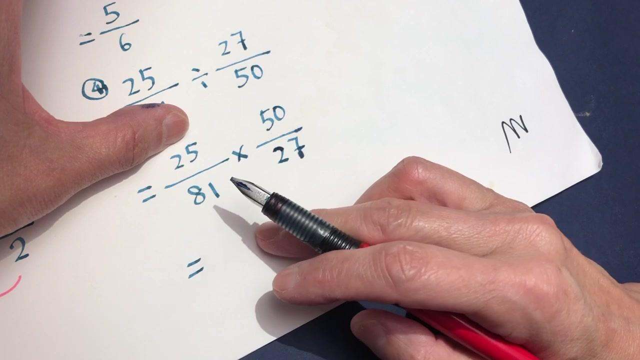 They are both the numerator. They cannot cross cancel. No matter how tempting it is, they cannot cross cancel. And eighty-one and twenty-seven, they are both on the bottom portion. You cannot cross cancel. This has to be. you have to time. 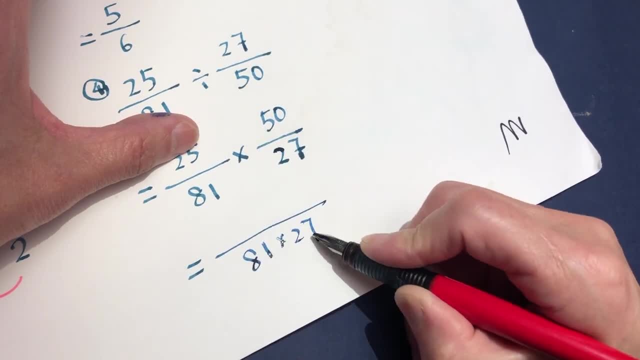 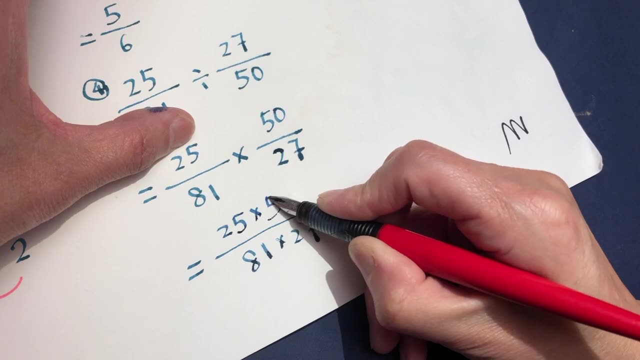 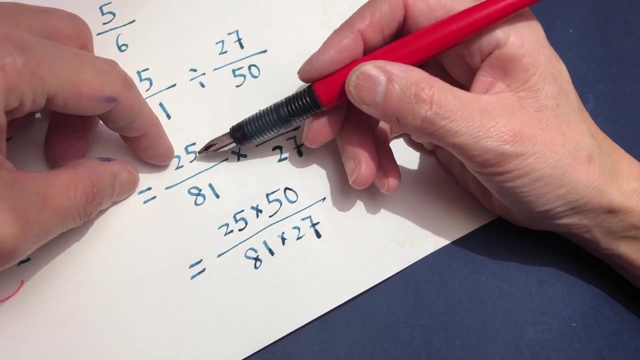 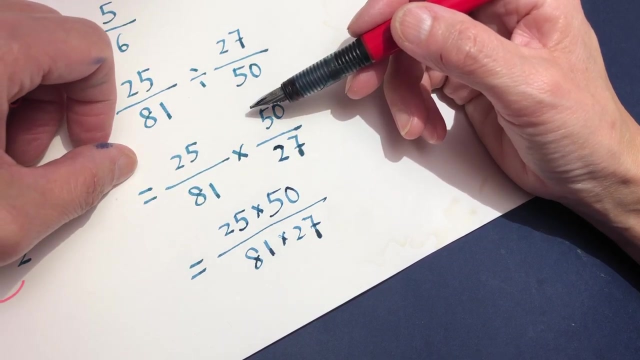 Eighty-one times twenty-seven and, on the numerator part, twenty-five times fifty. There is nothing you can do. You have to do this one, Because it's already to the simplest form. You cannot find common denominator, you cannot find common factors. 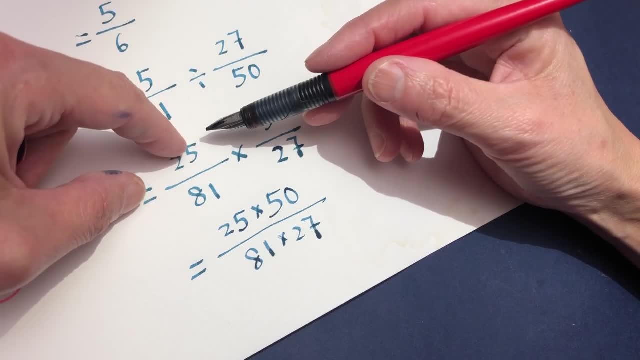 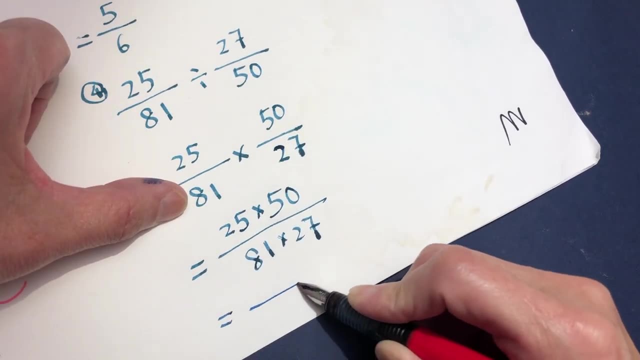 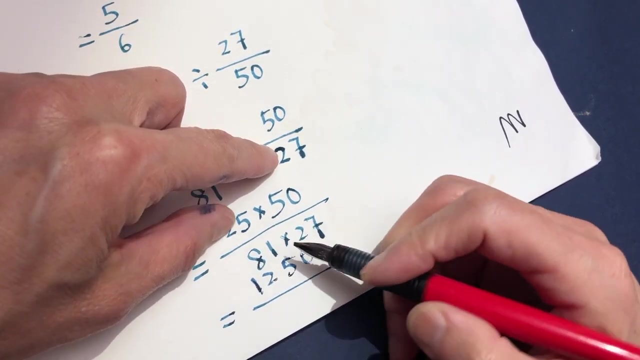 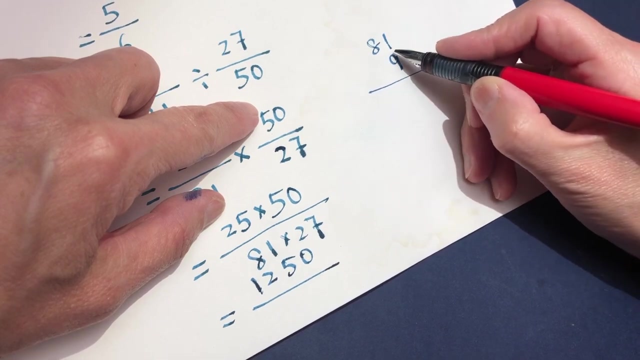 on the between the numerator and denominator, So you cannot do anything. So one hundred twenty is one, two five zero. eighty-one times nine. eighty-one times nine is, it's still three. Eighty-one times three is. 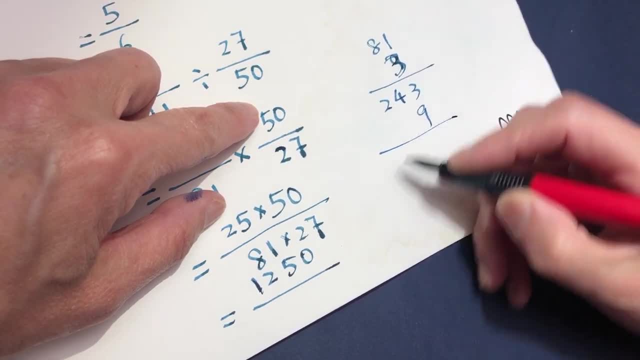 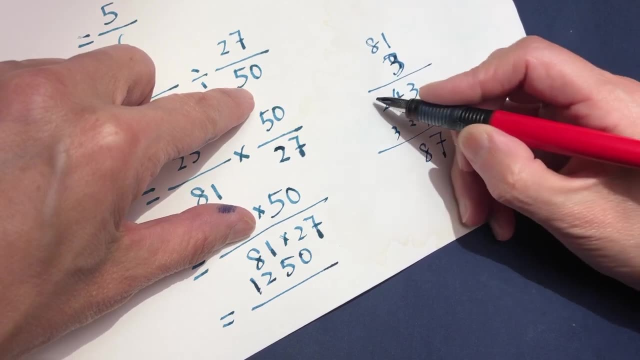 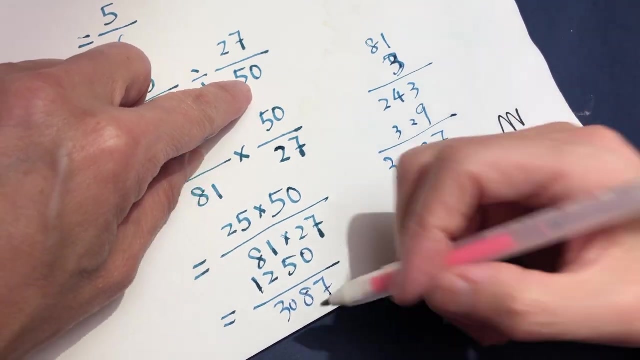 two, four, three times nine. three, nine, twenty-seven. four, nine, thirty-six, thirty-eight, three, nine, twenty-seven, thirty three, nine, twenty-eight, three, nine, twenty-seven. So this is the result. 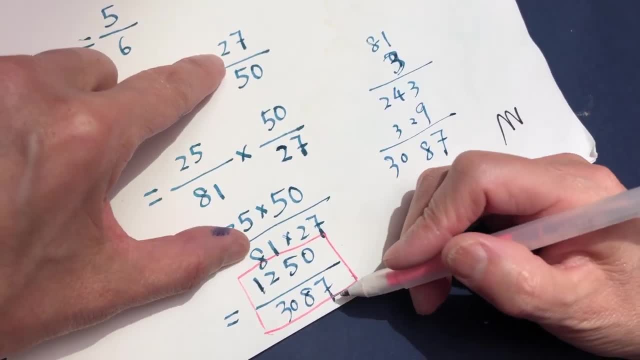 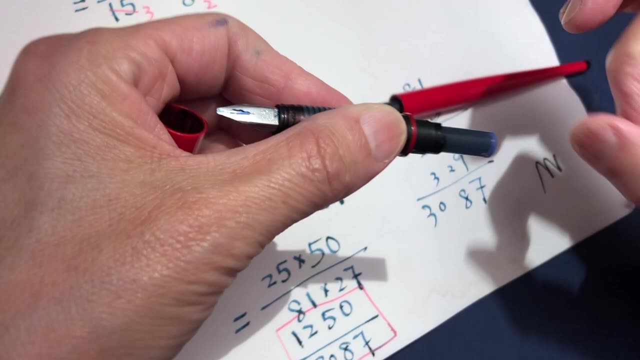 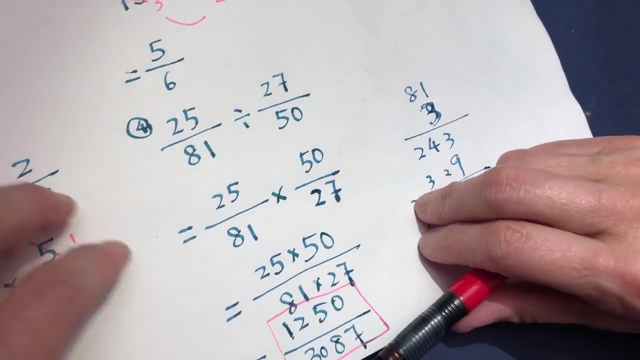 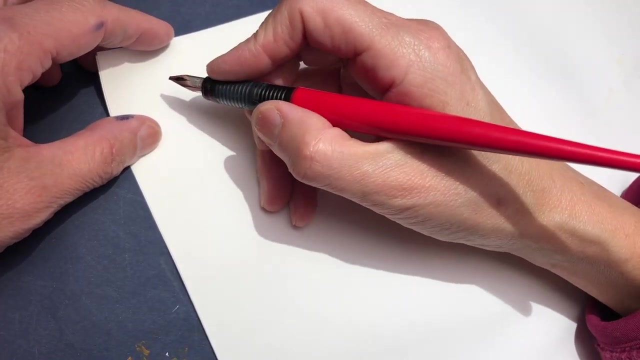 No matter how complicated it is, you have to do this. Okay, Now let's see. Maybe we will just stop here. No, We will do something of mixed number, Okay, So here we have one, two, three, four, five. 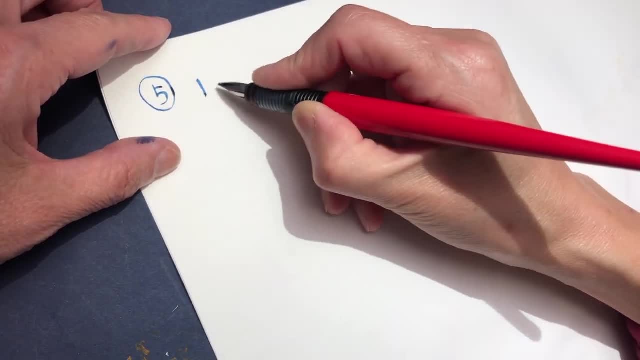 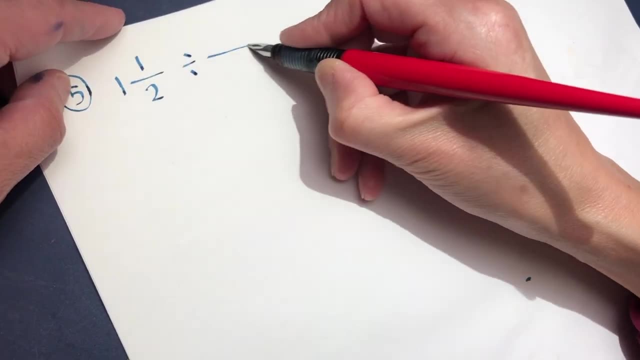 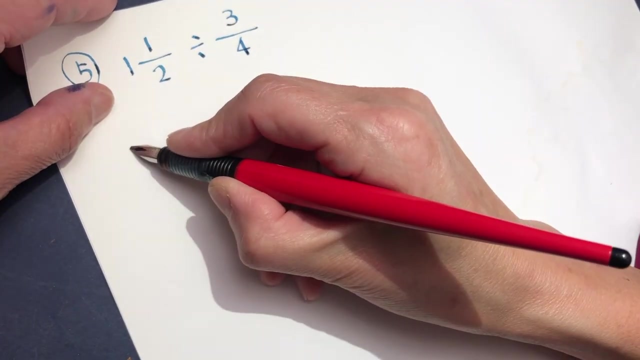 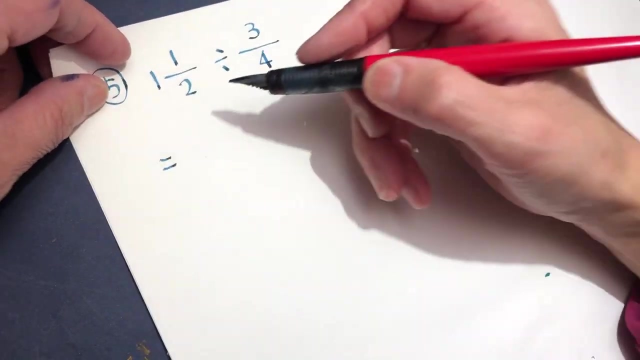 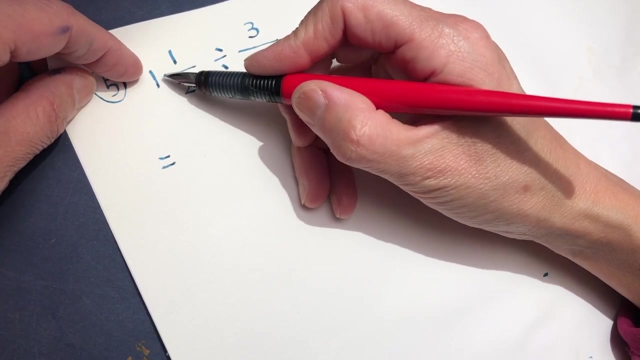 And this is a mixed number, One, and one over two, divided by three over four. What do we do? So the first one, the first, when we do multiplication and division, we have to change into pure factor form. It cannot be a mixed number. 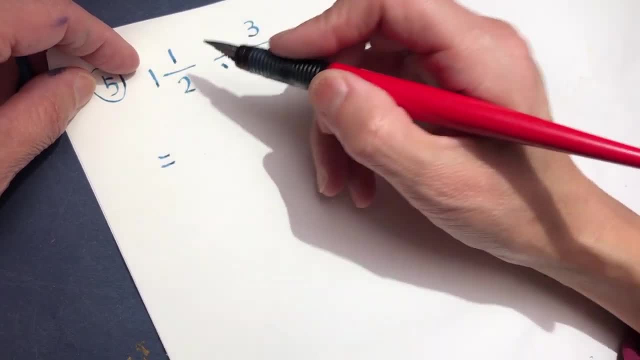 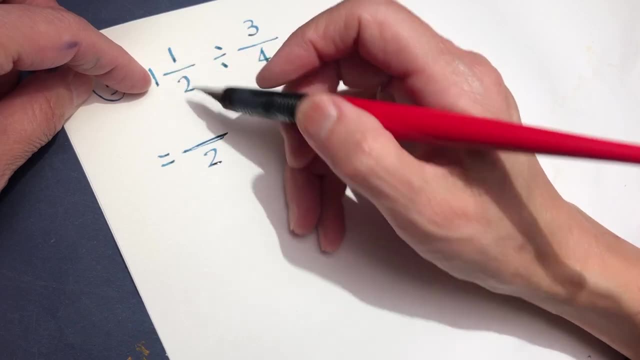 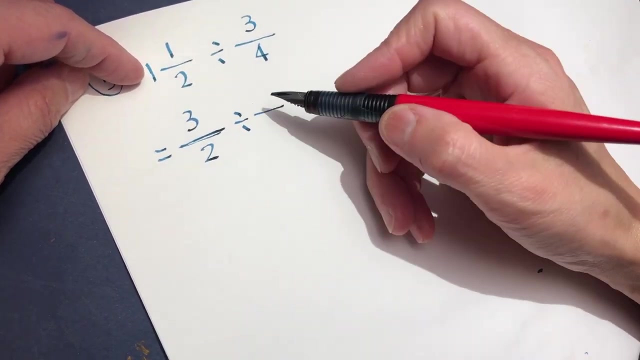 So we have to change it into a pure factor form. So the bottom, the denominator is two, The numerator two plus one is three Divided by. we will do it step by step. I will not change the sign yet. Three over four. 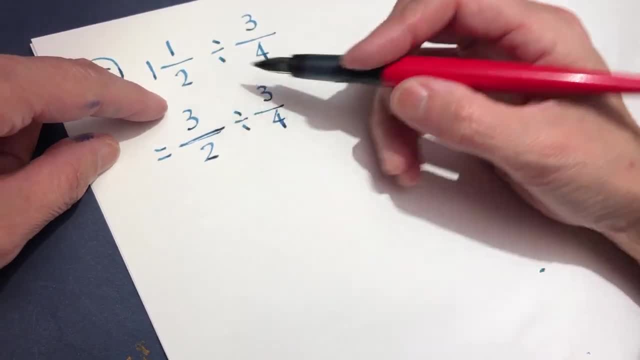 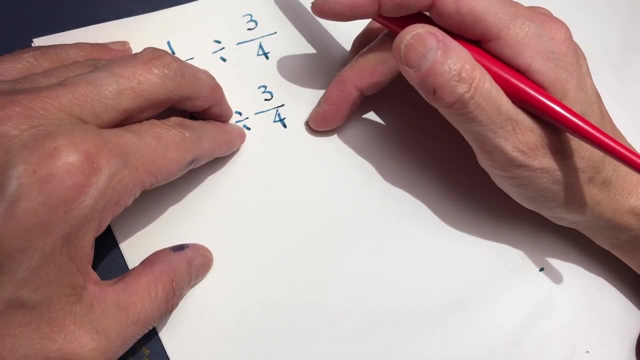 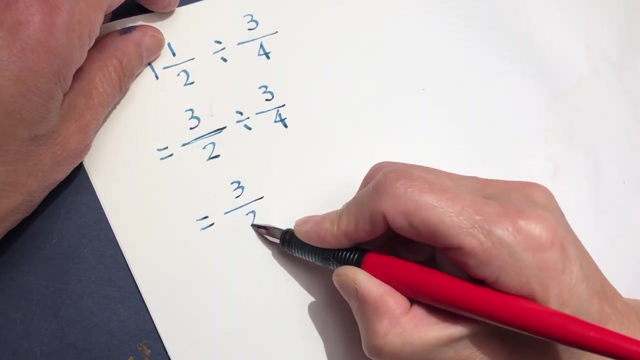 We finish one problem at a time. I know you can finish the second problem. No, we do not do it. First we change the first number, The second number, we just completely copy it, Do not change. And now, three over two. 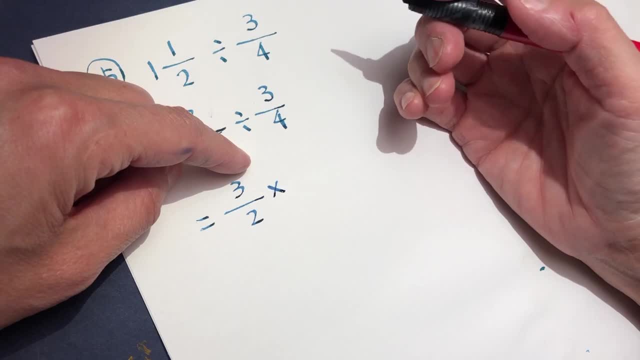 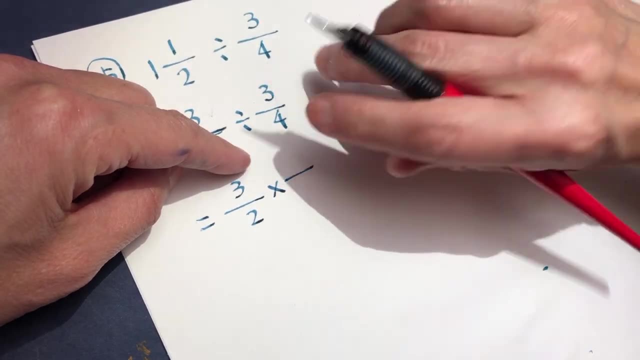 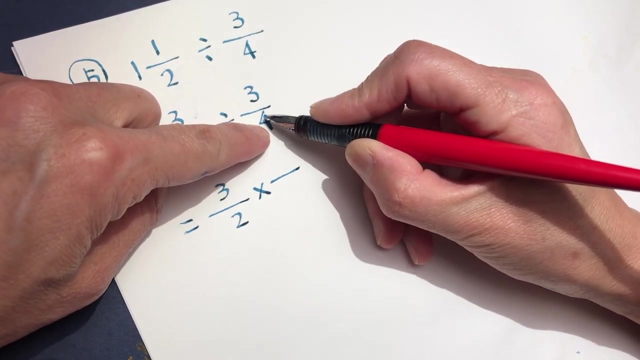 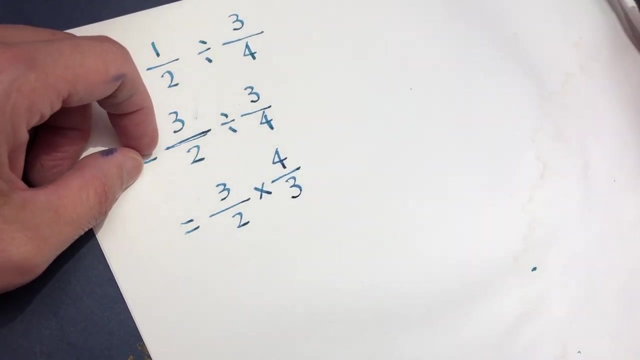 divide, we change into multiply. When we multiply we need to switch the number, Turn it upside down To time it's reciprocal. So four at the bottom. Now we move four to top And three to the bottom. This time we can use our glitter pen. 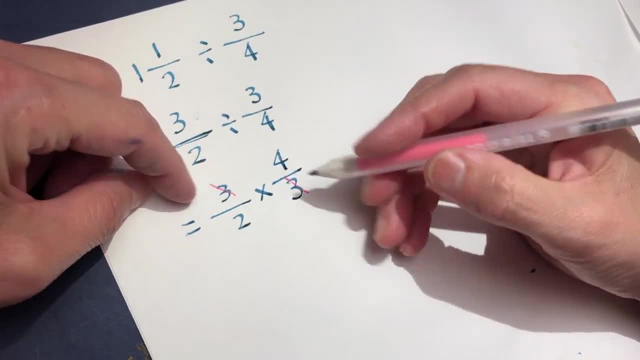 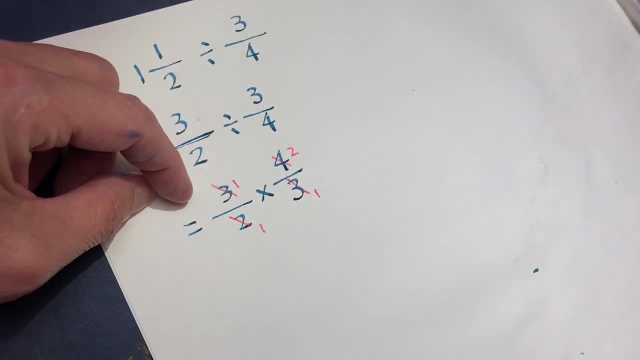 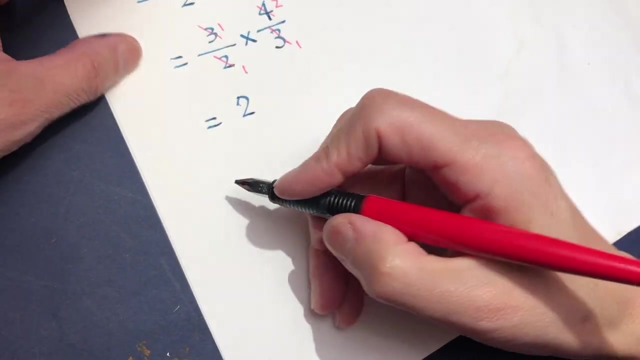 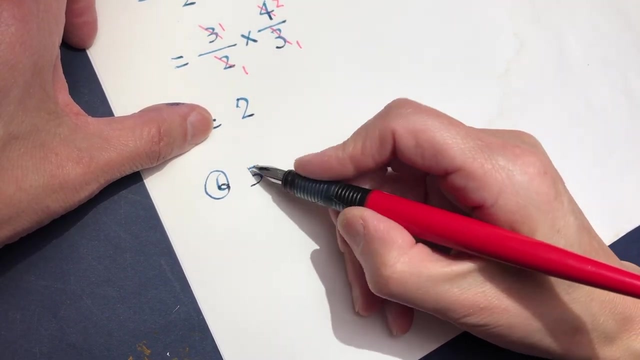 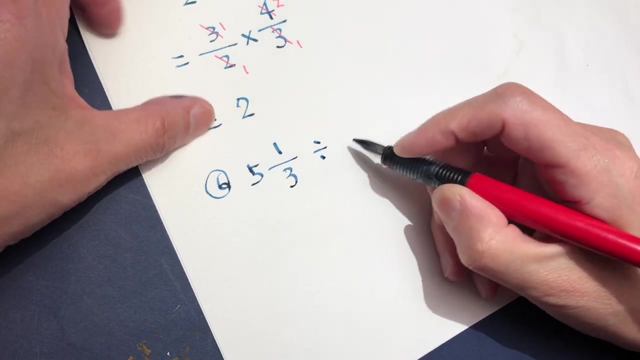 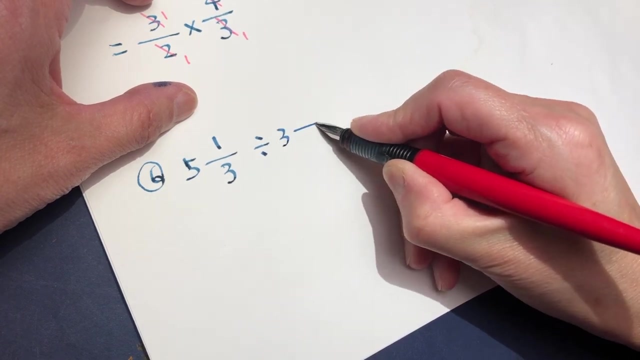 to cross cancel. Three and three become one And two, and four become one and two, And the result is two. OK, It's a little bit too simple, So let's do more complicated: Five and one over three divided by three and. 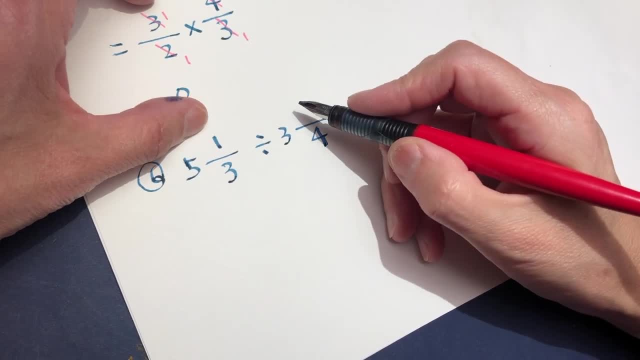 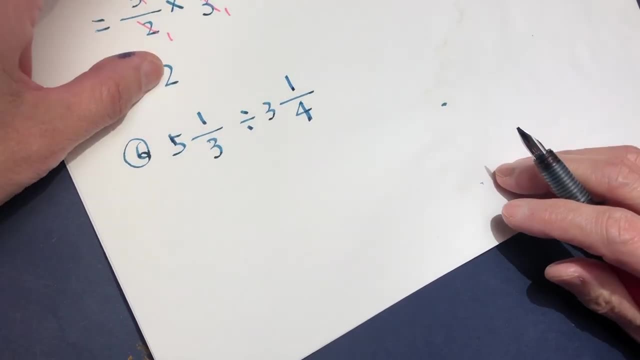 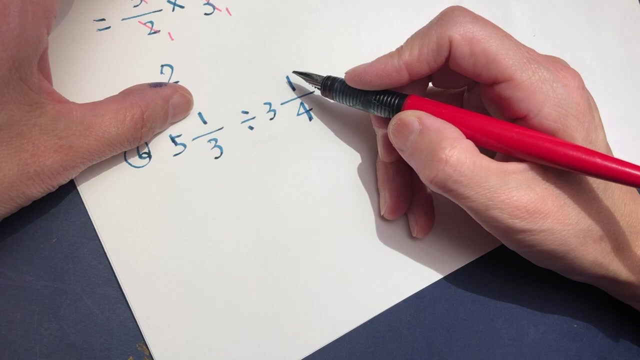 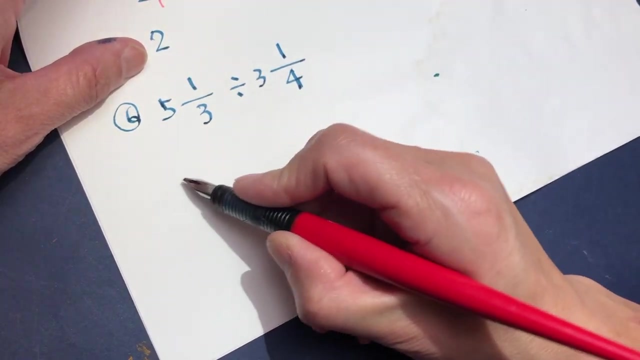 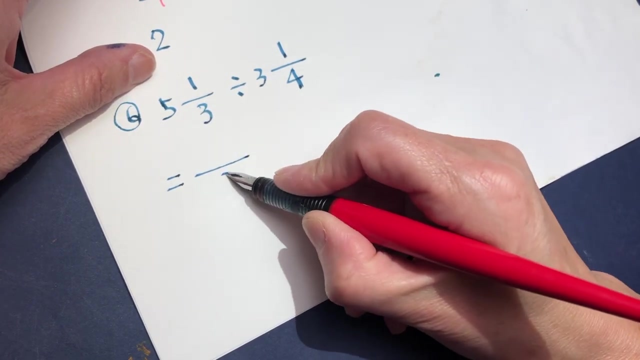 four over four over four over one, Four over three, Four over OK, Let's do it. It's not a very smart problem, but let's just do it. So five and one over three becomes three at the bottom. 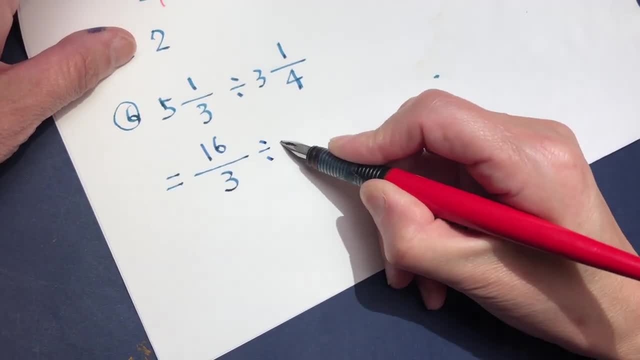 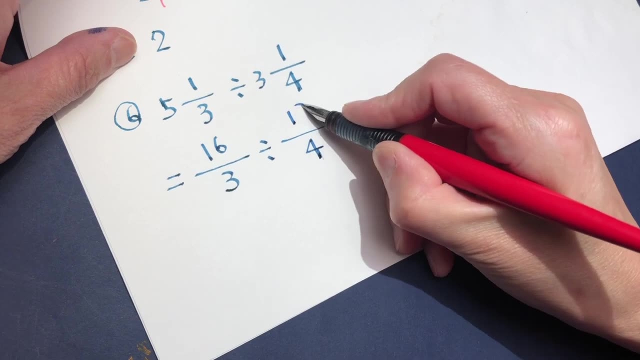 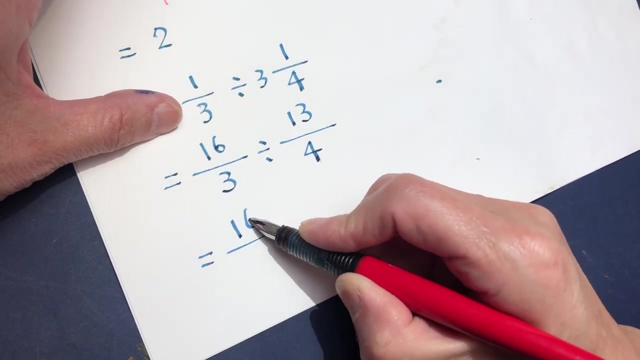 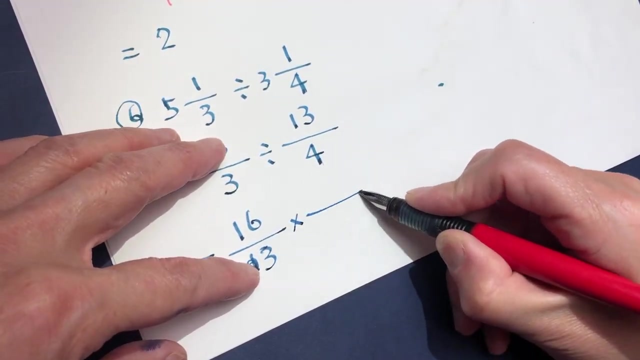 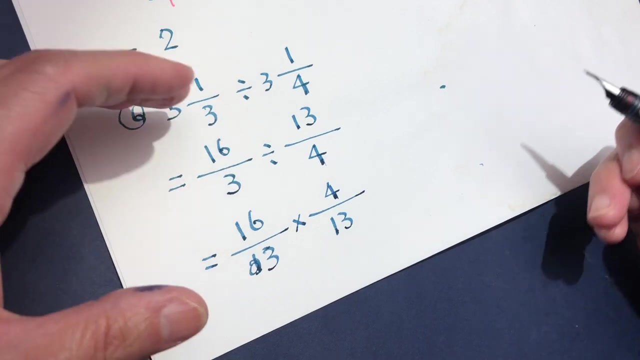 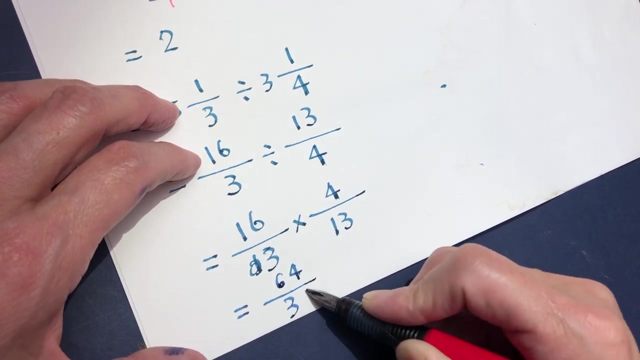 Sixteen over three divided by- since four is the bottom thirteen on top, equal to sixteen and three, Sixteen over three times thirteen, Four over thirteen. There's nothing we can do. It can be sixty-four over thirty-nine. You can do, just leave like this. 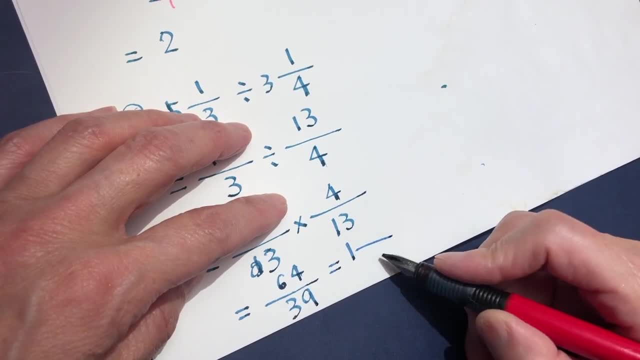 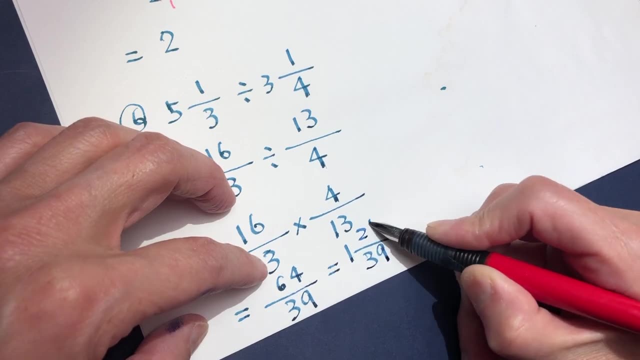 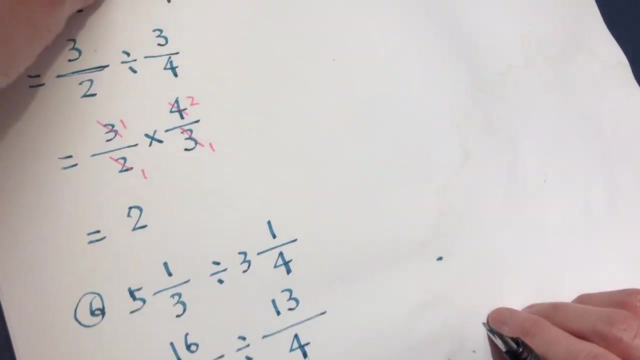 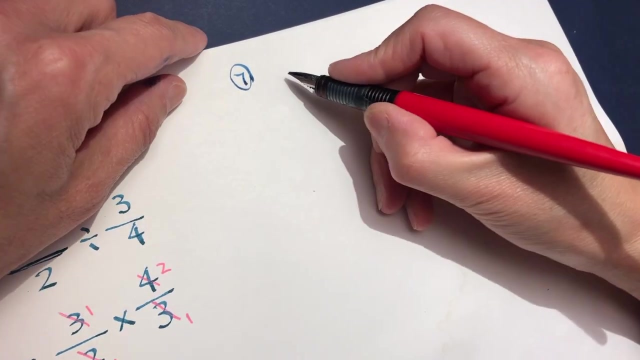 or you can change into into a mixed number form: Thirty-nine is twenty-five And thirty-nine, twenty-five over thirty-nine. OK, Number seven. we will try to think of a little bit smarter number. OK, Seven and one over three. 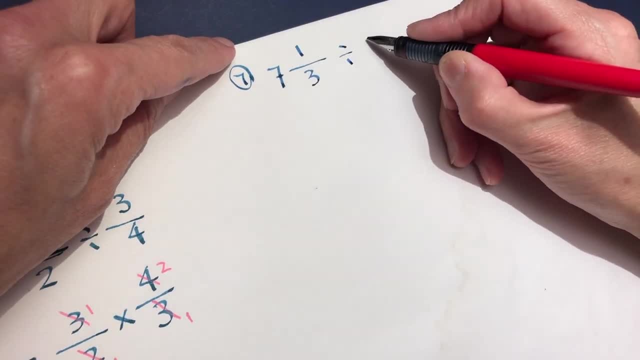 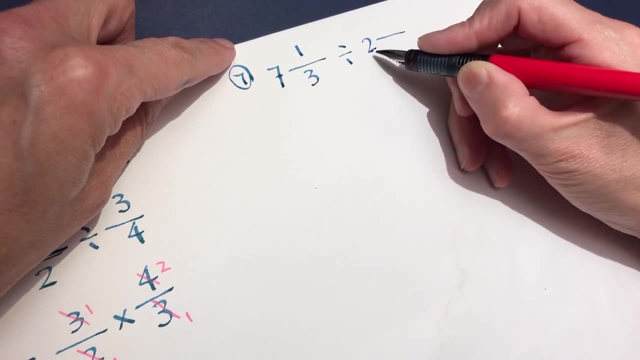 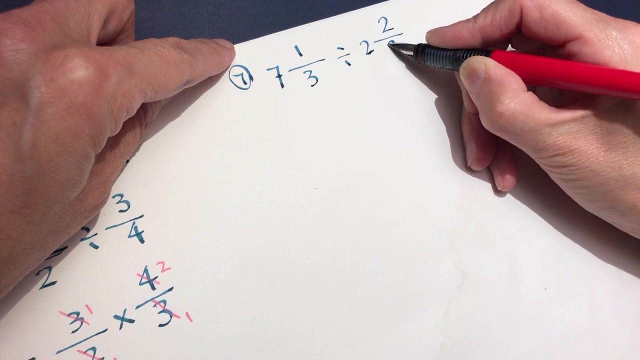 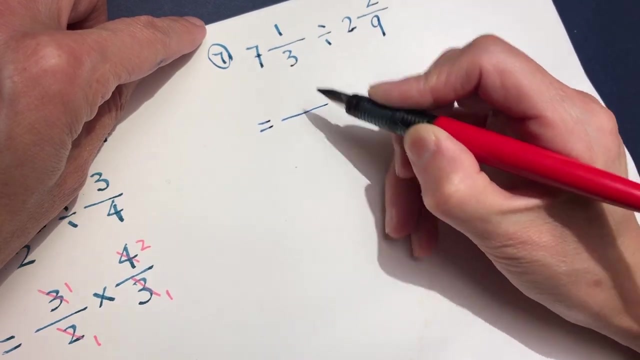 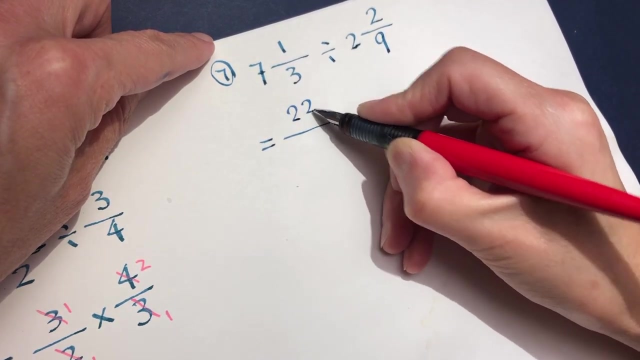 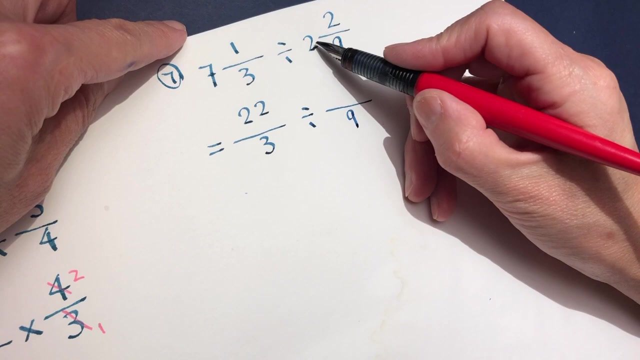 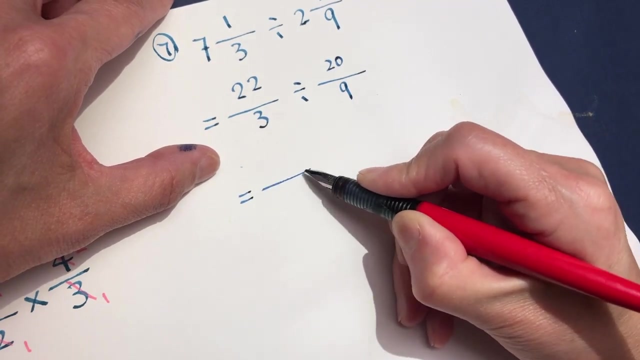 divided by two, and two over nine, Two and two over nine. This might be a little bit easier. So change first number into twenty-two over three. divided by nine is copying and twenty, And this time we can copy the first number. 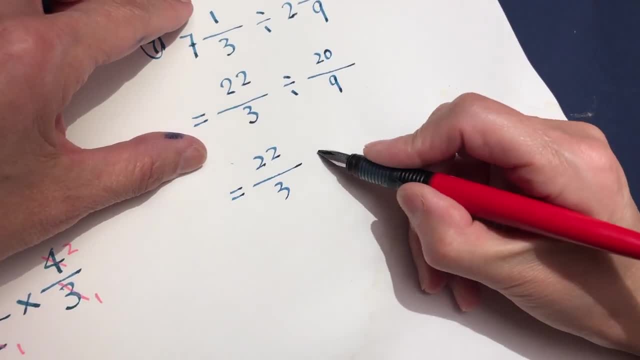 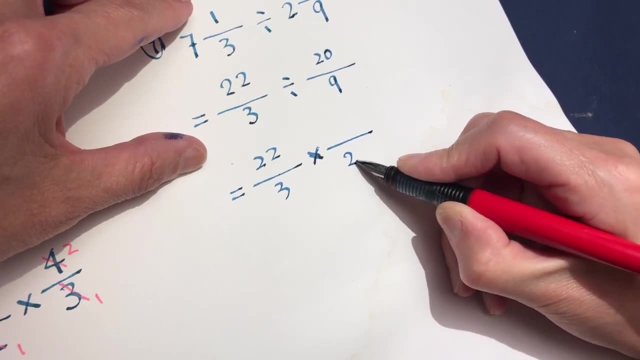 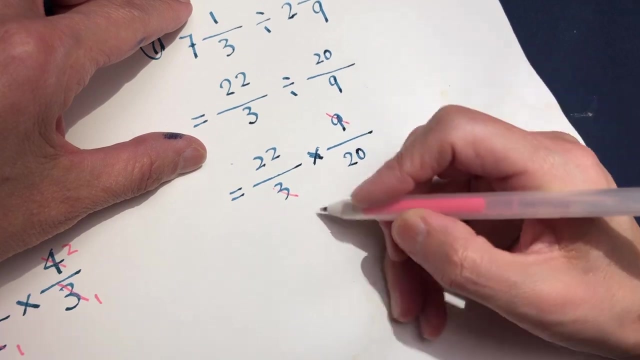 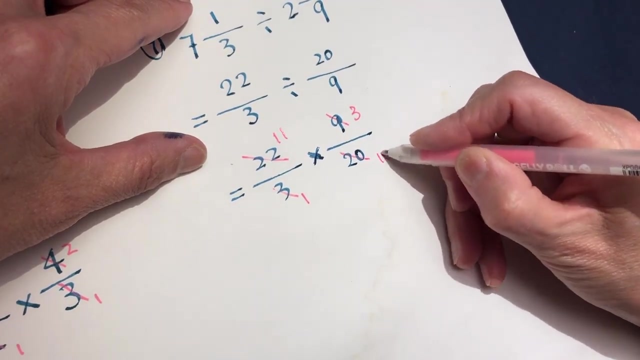 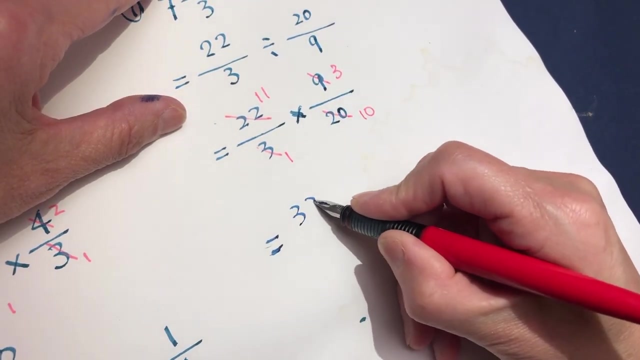 Do not change And the second number turn it upside down to change into multiplication: Twenty on the bottom, nine on top. Now we can use our glitter pen: One and three, And here is eleven and ten, So it becomes thirty-three over ten.